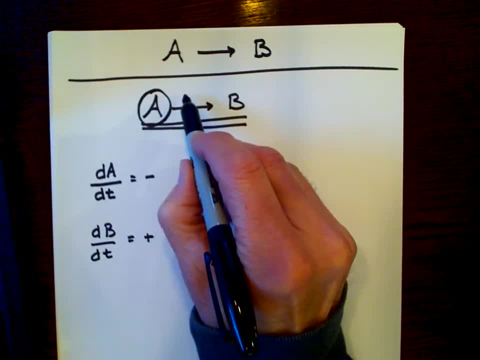 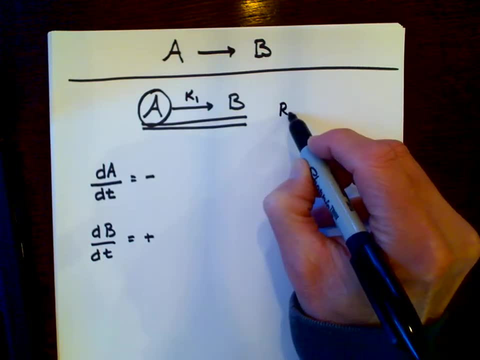 in the mechanism, in the mechanistic step, I should say, And we give each step a certain rate, constant, We'll just call this one K1. And so I would say, okay, well, the rate for this step is going to be K1 times the concentration of A. 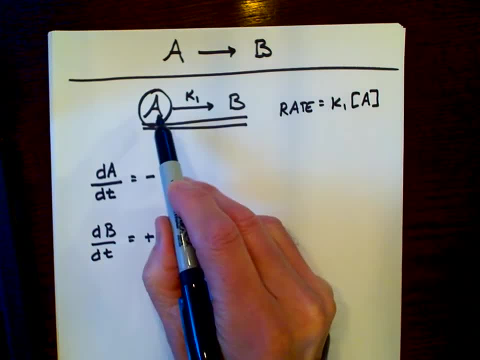 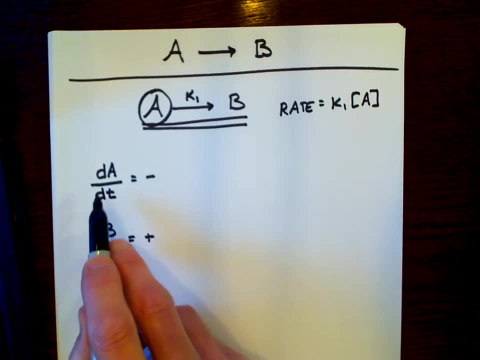 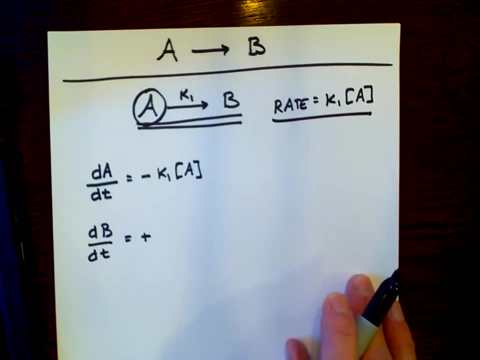 It will be A to the first power, because there's only one A molecule in the in the reactant side of this step, And so we'd say that dA dt is negative, K1 times the concentration of A, because that's our rate for this step, Whereas dB dt that's going to be positive. 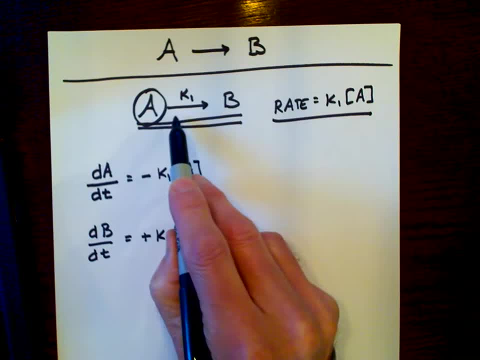 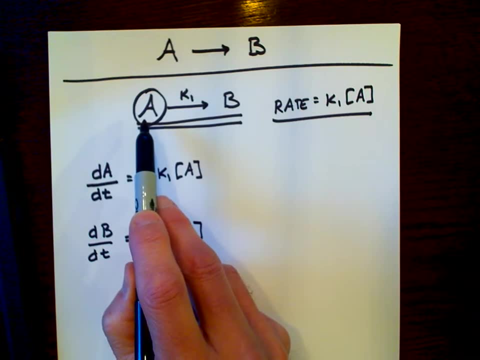 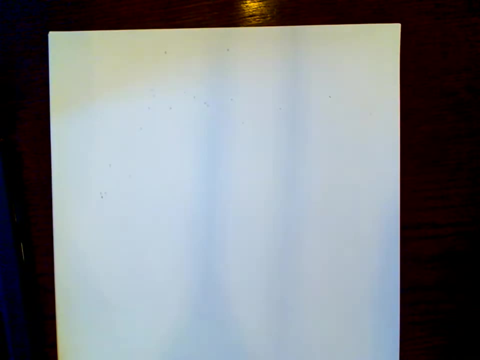 K1 times the concentration of A. So how fast B is accumulated by stoichiometry is going. It's going to be the opposite of how fast A is depleted. That's an easy case. It could be that this mechanism, however, 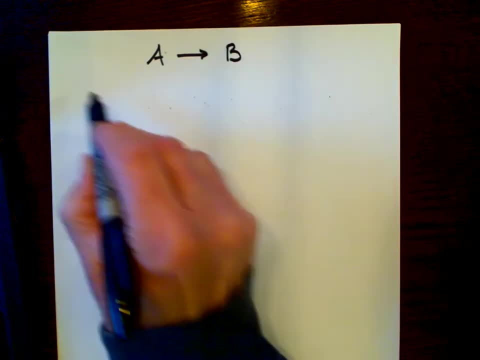 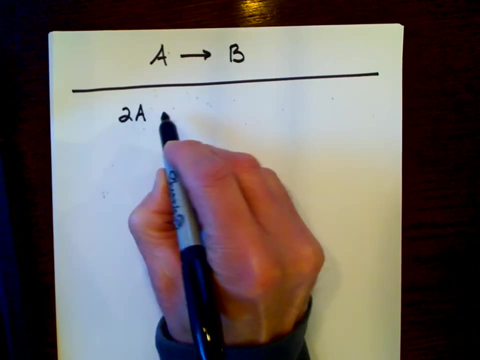 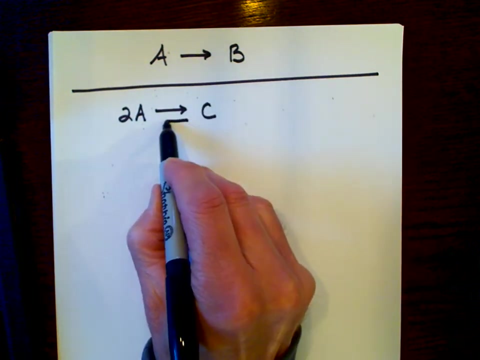 proceeds by a more complicated process. So let's just check this out. We could have, for example, in step one we could have two molecules of A going to some molecule C And we could also have that molecule C splitting up and going back to two molecules of A. 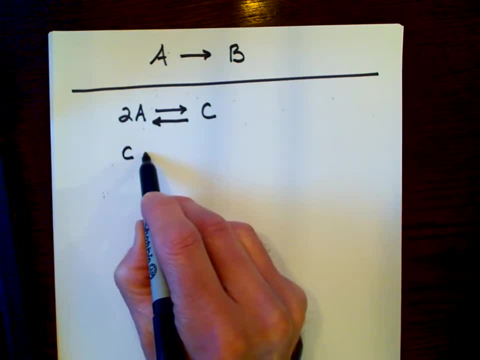 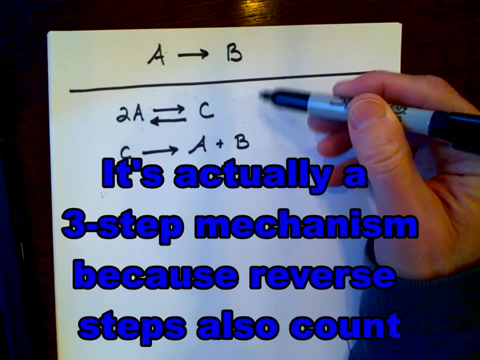 And then that molecule of C, once it's formed, can move on to form a molecule of A and a molecule of B. So we would say this is a two-step mechanism, And it's always the case that when we propose a mechanism, 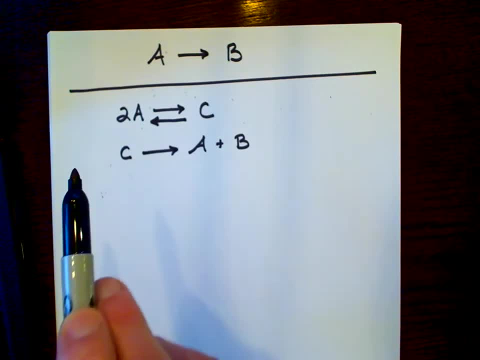 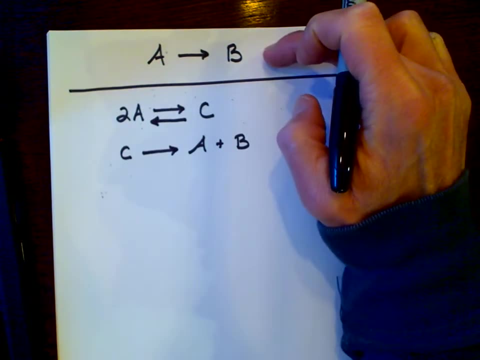 so in this case we have two mechanistic steps, and it's always got to be the case that our two-step mechanism is going to be the one that's going to. somehow we have to be able to add these together to get our overall reaction. 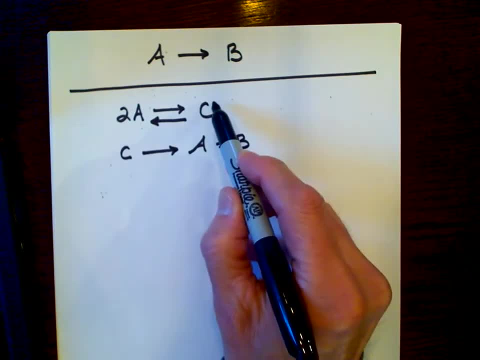 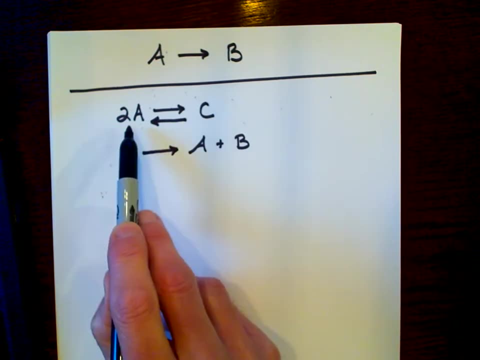 In this case it's quite simple: If we just add these two together, I'm gaining a C and losing a C, so that's a wash. And here I'm gaining an A and losing two A's, so that means I'm ultimately losing one A. 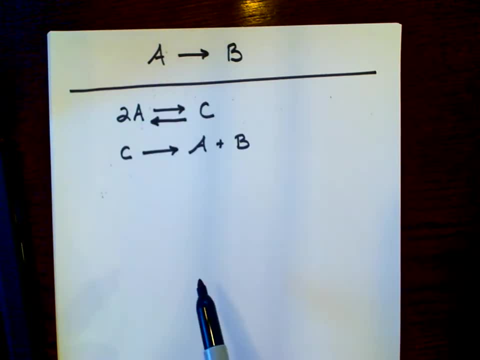 So if I add these two together I end up getting A goes to B. Now here the differential equations are going to be more difficult, because we have three species And we have three steps, And I'm going to name these steps: K1 for this: going in the forward direction. 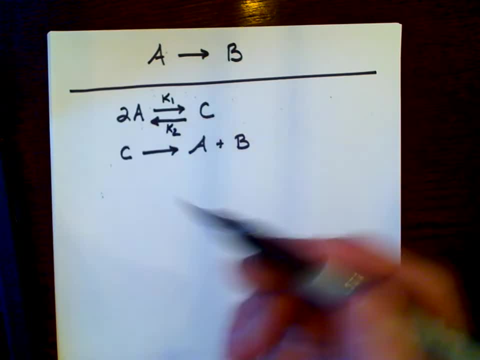 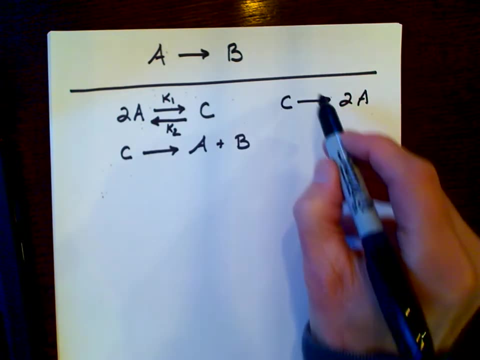 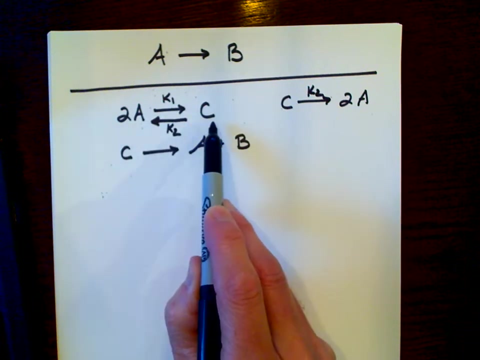 K2 for this, going in the reverse direction, which is basically C goes to 2A. I mean we could write this as three steps, right? We could just put this like this: Rather than writing this reverse arrow, we could just write: 2A goes at rate K1 to C. 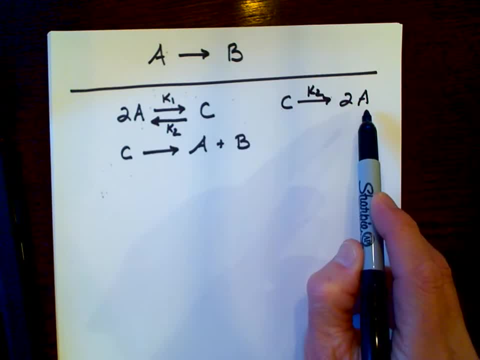 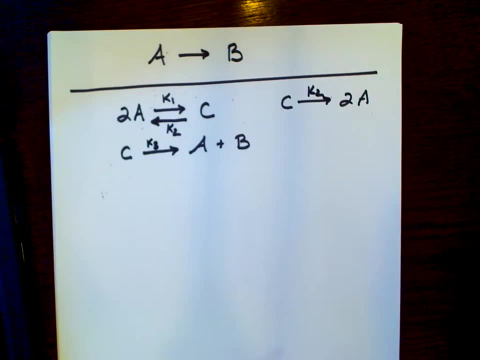 And then C goes at rate constant K2, back to 2A. And then, here, in our third step, C goes back to A plus B, so we're going to call this rate constant K3.. Now, what's going to be the change? 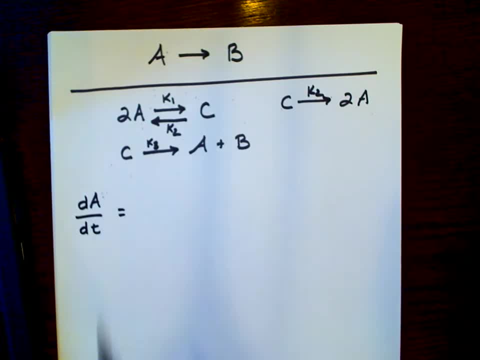 in the concentration of A with time. Well, if we look at step one, actually we should recognize that all three steps influence the concentration of A's, because in step K1, I'm losing A, In step K2, I'm gaining A. 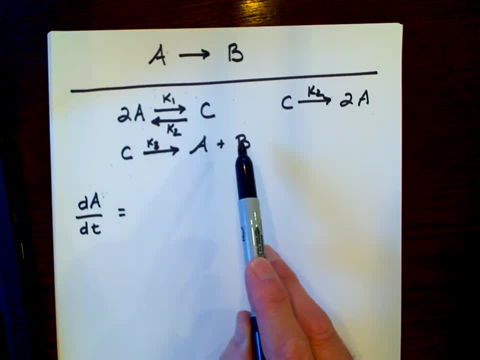 And in step K3, I'm gaining A. So let's see, Let's do this. So the change in A with time, let's see K1- is going to cause us to lose some A, so I'm going to write a negative K1. 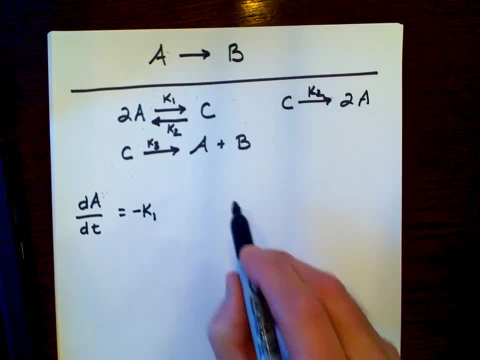 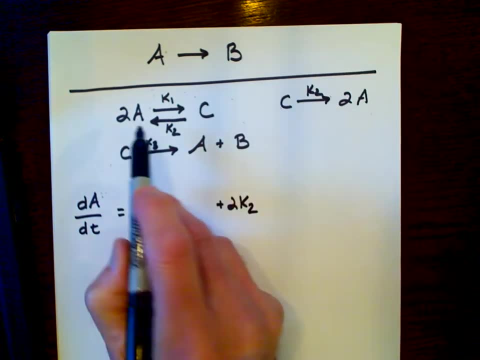 Step two is going to have me gain some A, and it's actually going to have me gain twice A, so I better put a 2K2.. And, of course, over here I'm losing 2A for every time this goes. 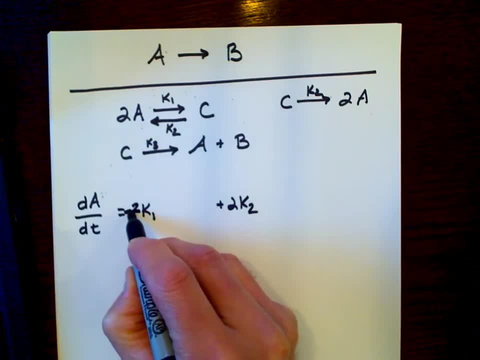 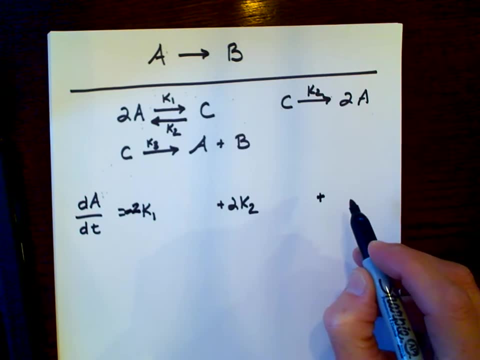 so I should have done a negative 2.. Sorry, that's a little messy, but a negative 2K1 for this step And then in step three, for A, we're going to have a positive K3 because in the third step we gain A. 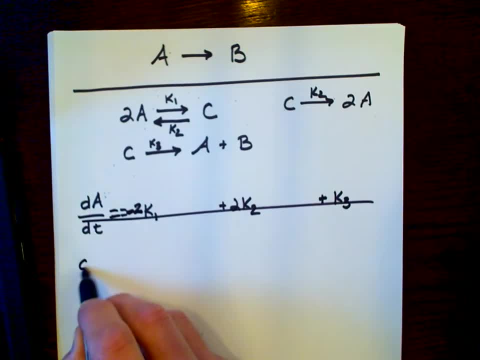 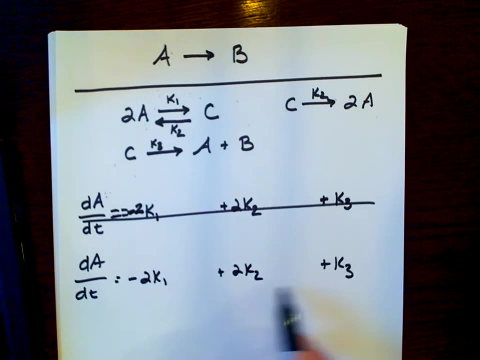 All right, that's a bit messy, Let's just rewrite it. So DADT is going to be a negative 2K1 plus 2K2 plus K3.. Now, what are the concentration dependencies of these steps? Well, if we look at step K1, which is in this direction, 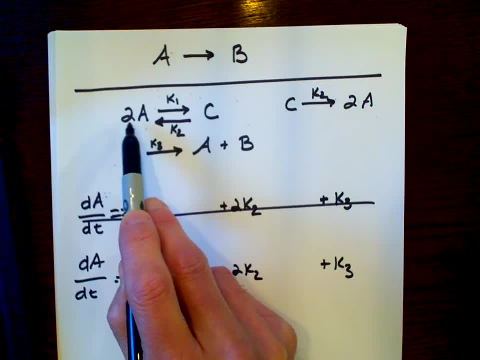 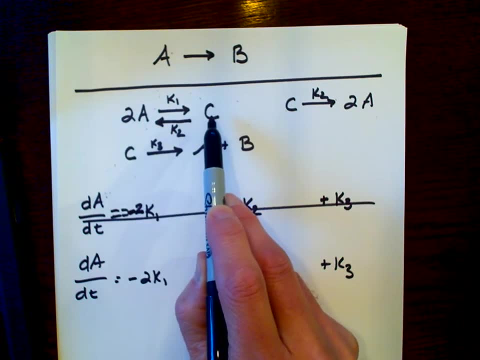 in step K1, the reactant's A, but there's two of them, So two A molecules have to collide in order to form a molecule of C. So because of that, this step is going to be dependent on the concentration of A to the second power. 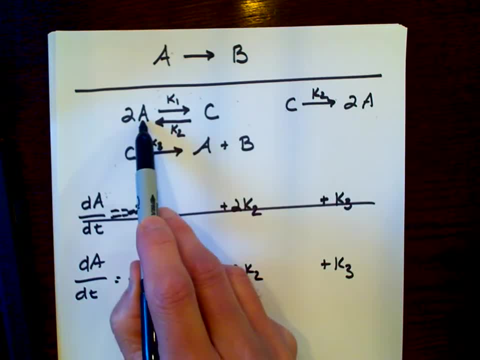 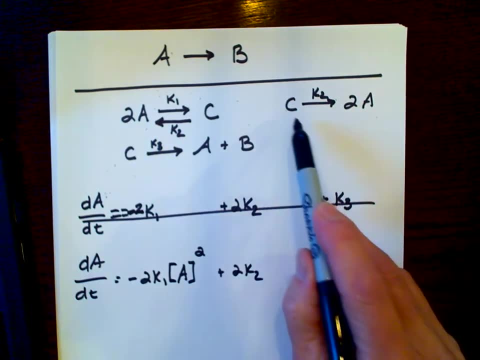 So this is always going to be related to how many reactant molecules are colliding in each case. For step K2, the reaction is driven by how much C is present, and C alone, And so step K2 will be based on the concentration of C. 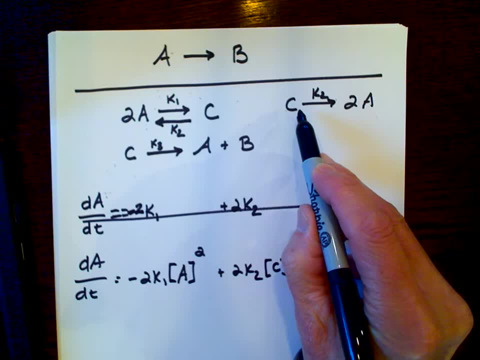 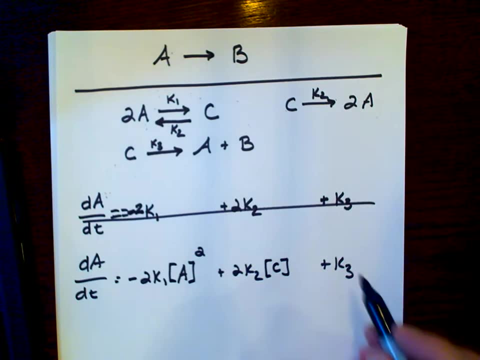 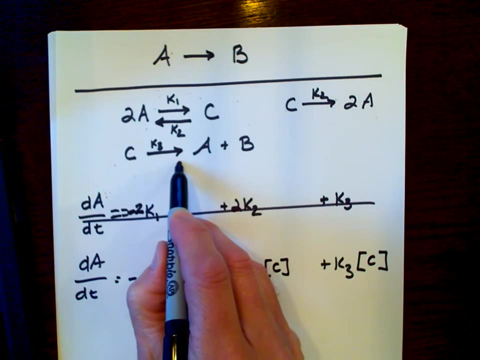 to the first power, because there's only one C molecule And then step K3, that's also going to be dependent on the concentration of C- to the first power. So we would write it like this And just to show you if there was a reversible step here. 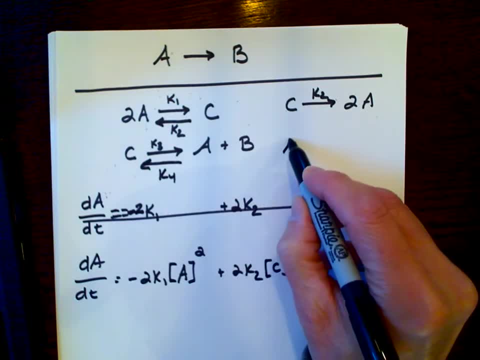 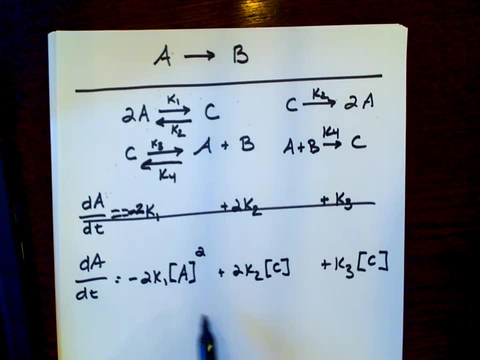 where A plus B goes back to C, we'd call that K4.. We could write it like this: A plus B goes back to C in step K4. In this case we'd have to add another term for DADT. 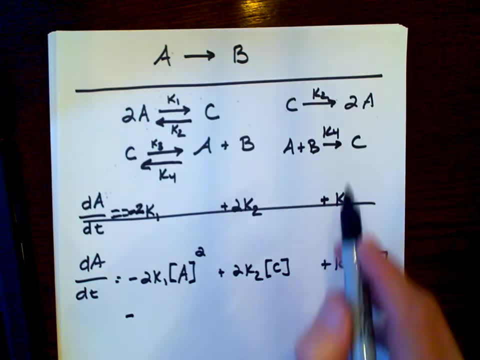 and that would be. let's see, we're losing a molecule of A in this step, so I'd put a negative here. It's going to be based on rate constant K4.. It's only one A that we're losing, so I don't put a two out in front or anything like that. 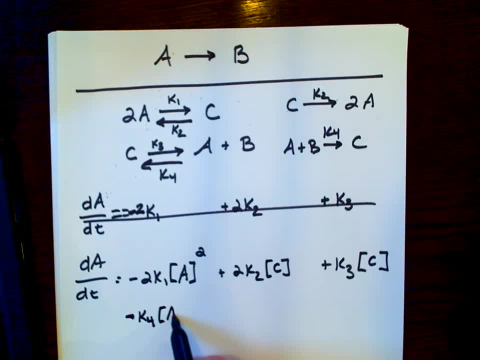 And then the concentration dependence. on this step it's going to depend on both the concentration of A and the concentration of B, because one of these collides with one of these in that particular step. All right, So that would be. there'd be four terms. 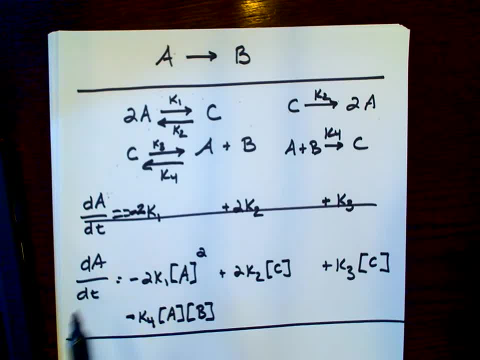 There'd be four terms for the change in concentration of A with time. And if we look at this, we see that there's in K1 we're flowing away from A, so we're losing A. So that's our first term. In step two, we're gaining A. 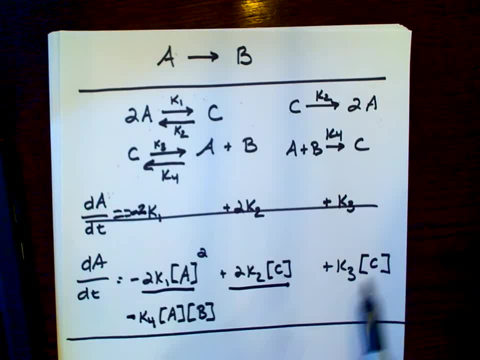 So that's our second term. In step three we're gaining A, so that's a positive K3 for our third term. And then in step four we'd be losing A, and so there's a negative term for that one there. 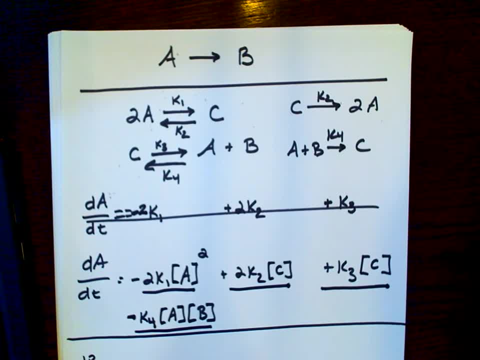 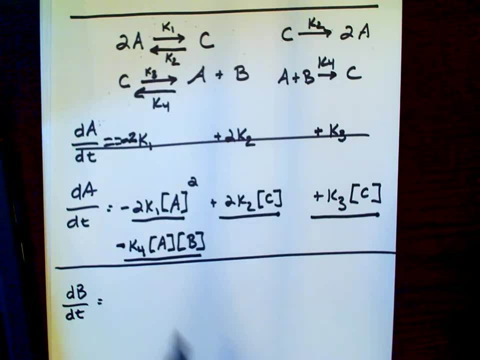 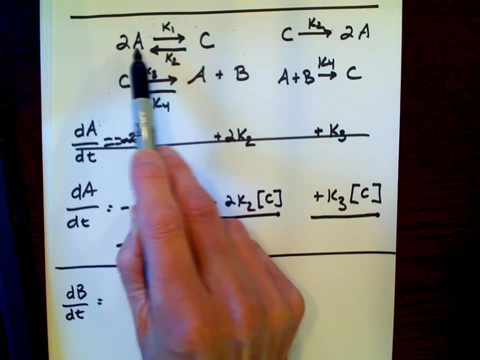 Okay, let's look at dB dt and see what that would be. So dB dt, based on our concentrations, we're going to say, okay, step K1, we have two A's going to a C B is not involved in this, so we don't include a K1 term. 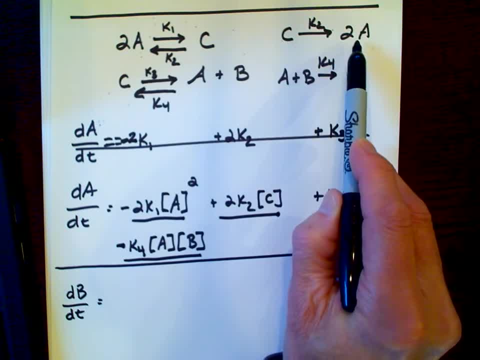 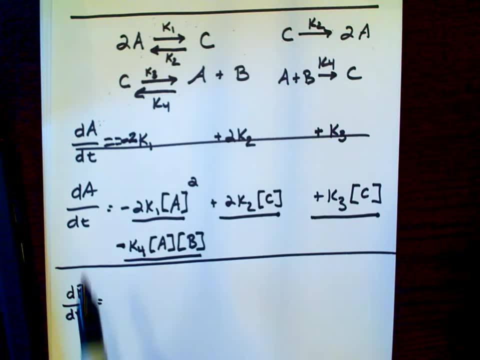 The second term we have C. going back to 2A. Again we don't have B involved, so we don't have a K2 term for dB dt. We do have a B involved in steps K3 and K4.. In step K3, we're gaining some B, one molecule of B, so we're gaining it. 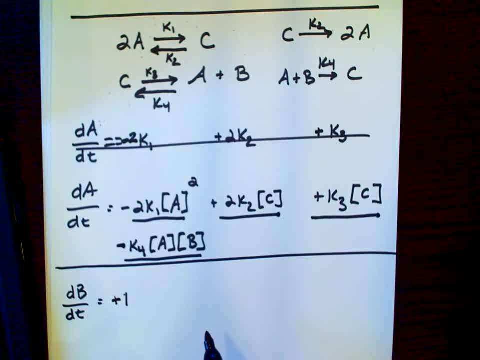 How many We're gaining one. I can write the one in here, just for emphasis. It's being run at rate constant K3, so it's 1K3, and we're going to write this based on the concentration of C, because this reaction 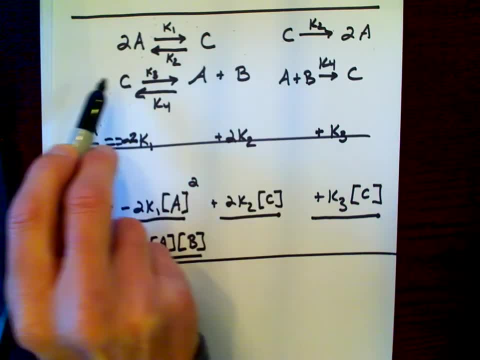 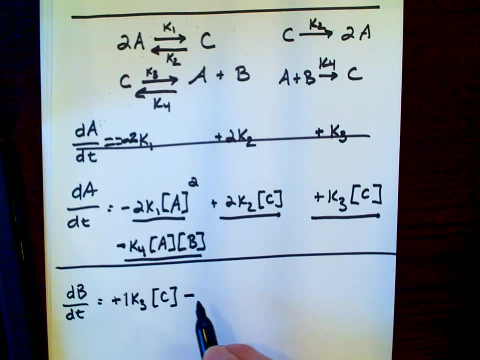 in the forward direction depends upon the reactants over here that are running in this direction In step K4, we're going to lose a single B, so I'm going to write negative K4.. Don't need to put the one out in front. 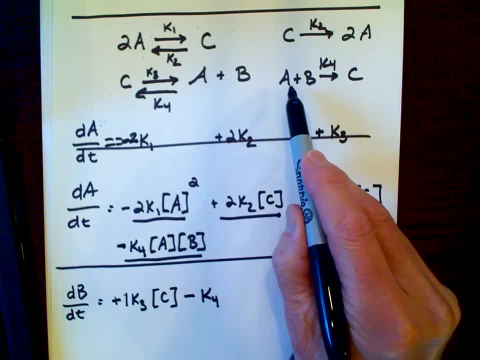 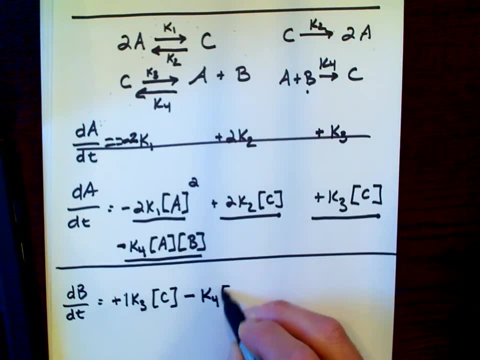 And then we're going to be running this. It's going to be dependent on the concentration of A and the concentration of B, both to the first power, because those are our reactants here. So it's going to be AB like that. 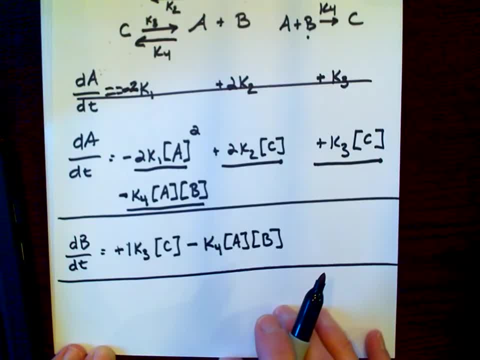 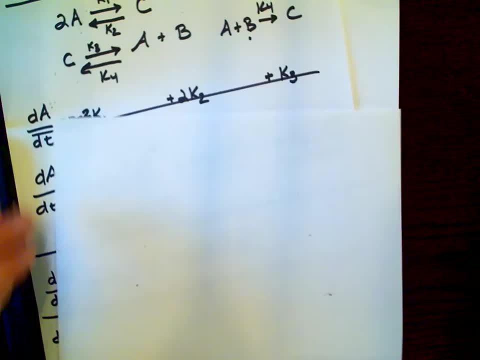 And then, finally, if we were going to run dC dt, this one might be a little hard, because I don't know where. Let's do it like this, Let's do it like this. Okay, here we go, We can run dC dt like this. 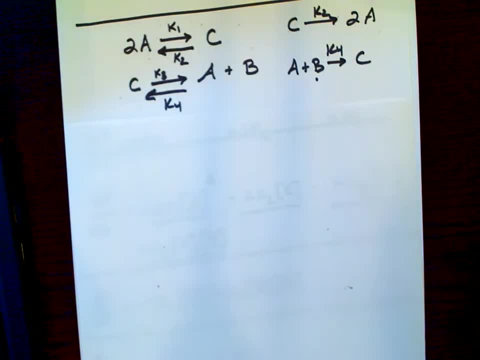 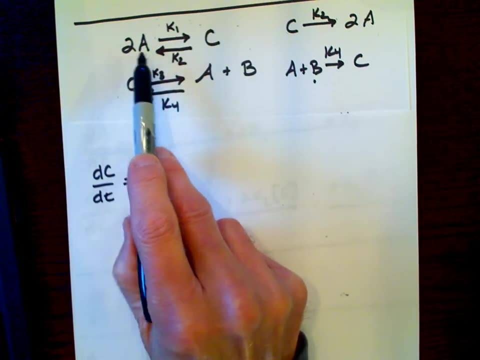 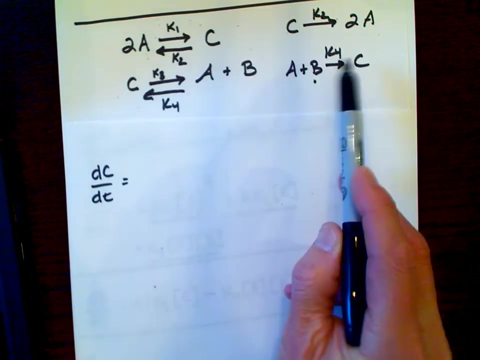 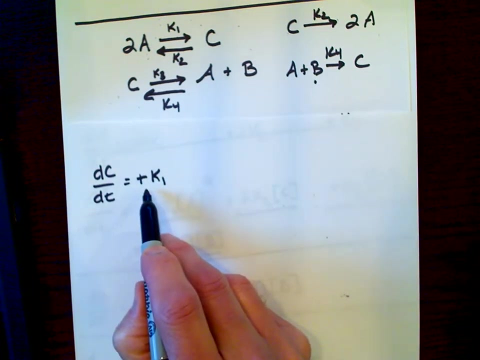 All right, dC by dt. let's see C is involved in step K1, it's involved in step K2, it's involved in step K3, and it's involved in step K4. It looks like it's gained in the K1 step and in step K1, that's going to be dependent. 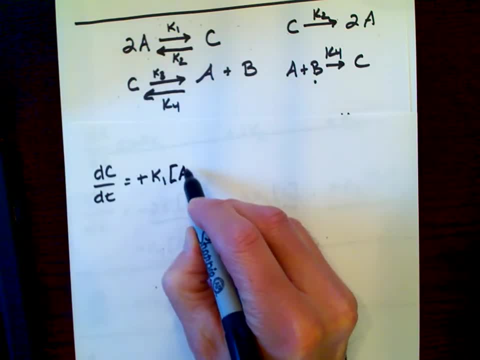 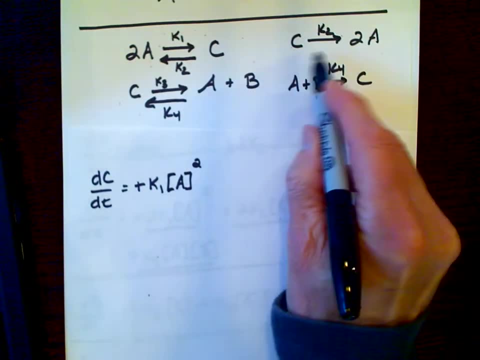 upon two molecules of A colliding. So we're going to need to do that. We're going to need to write A to the second power. The next step here. let's see we're losing C here, so I've got to write a negative K2,. 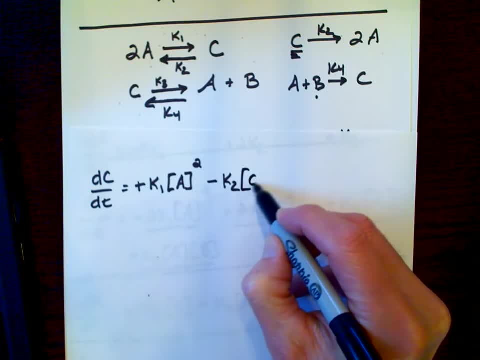 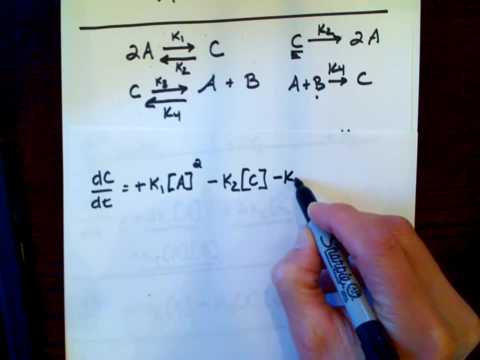 and that's dependent upon C to the first power. And then in step 3, it looks like we're losing C, so I've got to go negative K3 there, and that's dependent upon C to the first power, just the reactant. 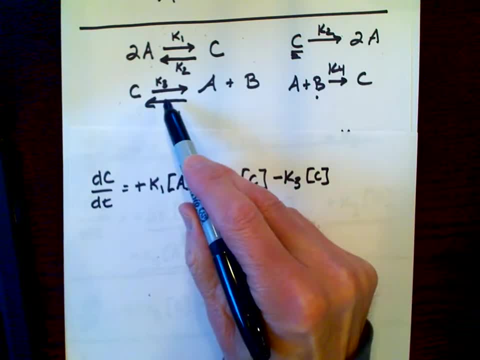 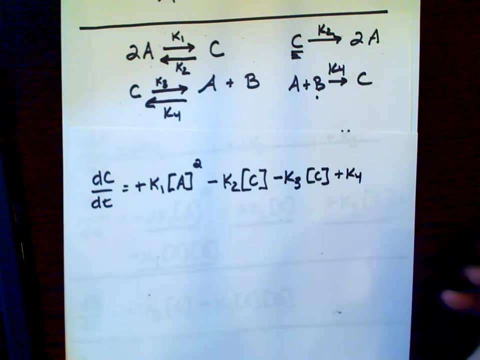 And then for the reverse step, which we can of course write like this: A plus B going back to C, we're gaining C, and that's going to be dependent upon the concentration of A to the first power and B to the first power. 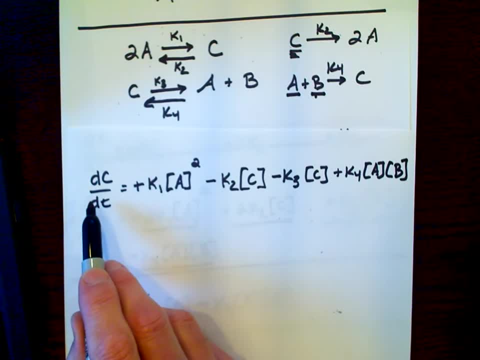 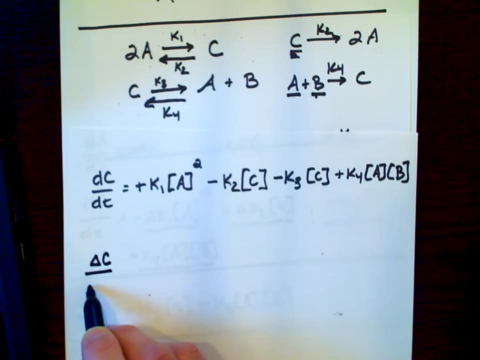 And then if I was running this in Excel. you know we can't do infinitesimally small changes in Excel, We can only do incrementally. So instead of DC DT, we change that to the change in the concentration of C over the. 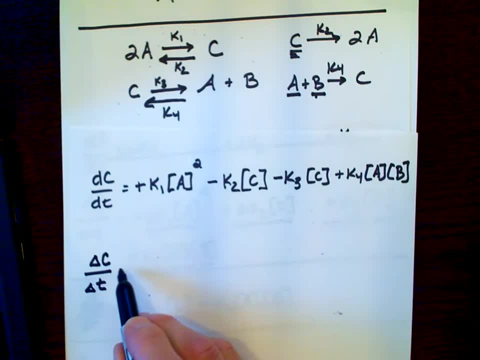 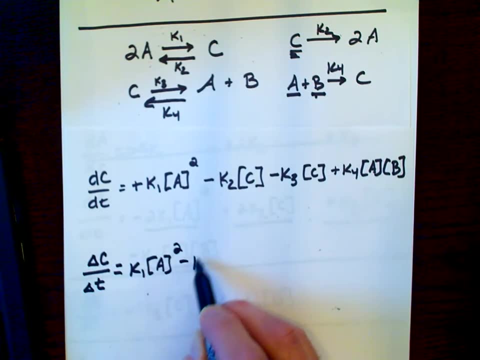 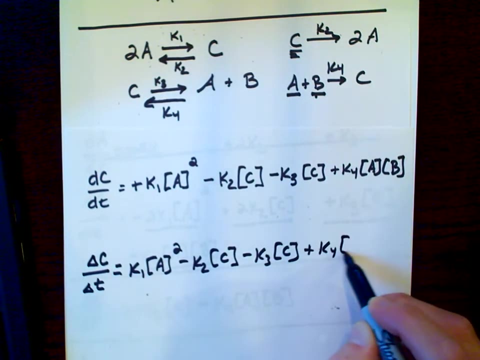 change in time. And so, for each subsequent step, well, let's just write it here. You know, this would be the same K1A squared minus K2C, minus K3C, plus K4AB, And what we do is multiply both sides of this by delta T, whatever we set our incremental. 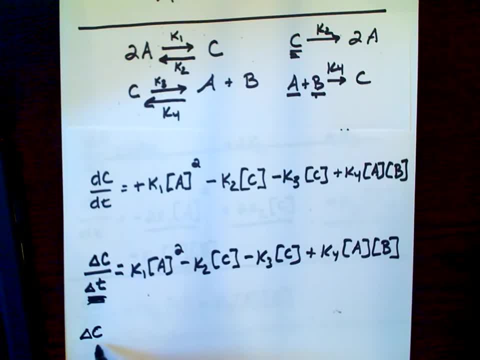 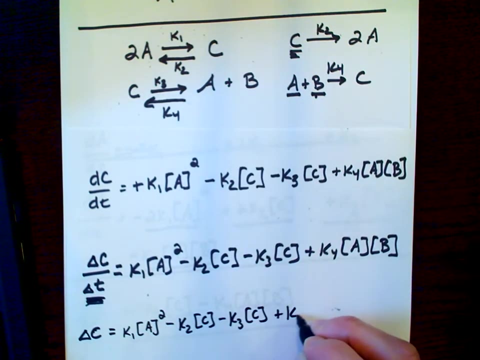 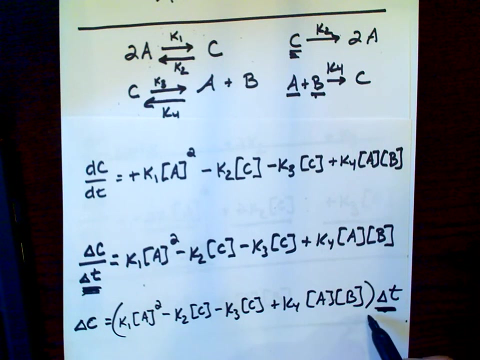 time unit to. So our change in the concentration of C with every time increment is going to be this very large- well, I should say four-term expression- All of this multiplied by The time increment that we choose And by squeezing this time increment down as small as possible, you know, then we approach. 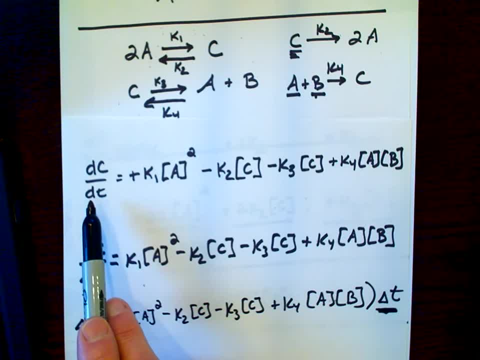 better values because, of course, we're getting closer to infinitesimally small unit change in time. The issue with that in Excel is that it takes a long time, a lot of rows to calculate. The smaller you make this delta T, the more rows it's going to take for you to calculate.